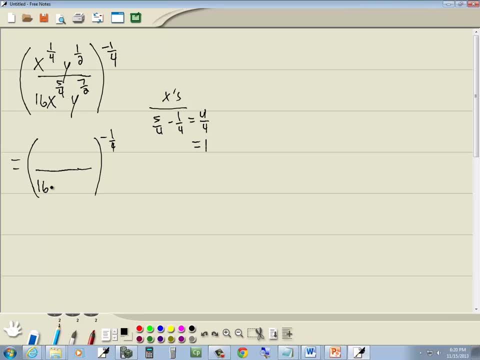 So we're going to have x to the first power where our larger exponent was, which was down below right. there Now the y's. We're going to subtract a smaller exponent from a larger one. So we've got seven-halves minus one-half, which gives us six-halves, and six divided by two gives us three. 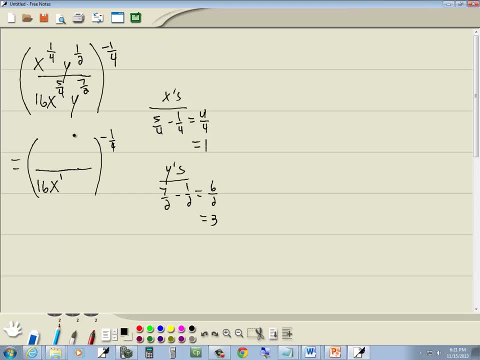 So we're going to have y to the third power, where our larger exponent was, which was down below, And then we'll put a placeholder of one up there. If everything disappears in a fraction, then you always have a one there by default. 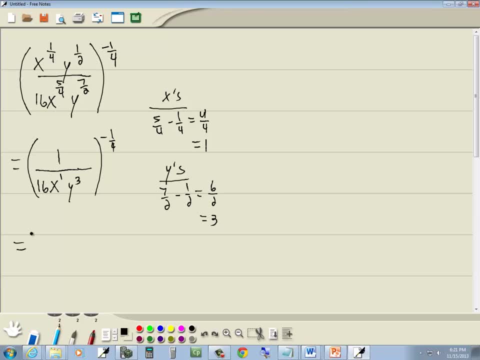 Okay, there's nothing left to do inside the parentheses. So notice, Notice, we have a fraction to a negative power. So we're going to flip the fraction. take a reciprocal of it. This becomes sixteen: x to the first, y to the third, over one. 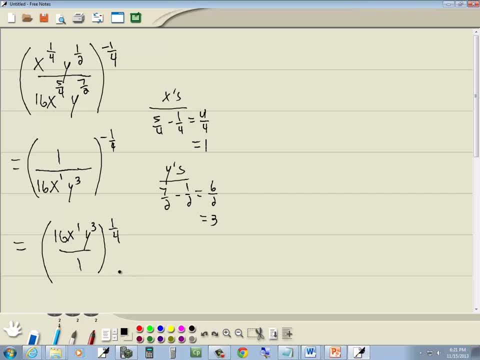 And then you change the sign of the exponent. It becomes the one-fourth power. Okay, well, that one can drop away. So that just gives us sixteen x to the y, Sixteen x y to the third, all of it raised to the one-fourth power. 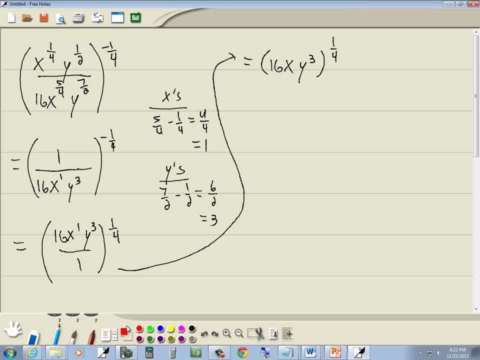 Now, if everything inside of your parentheses is either multiplication or division and you're raising it to a power, then you can take everything to that power. It's kind of like a distributive property concept. So we're going to take the sixteen to the one-fourth power. we'll take the x to the one-fourth power. 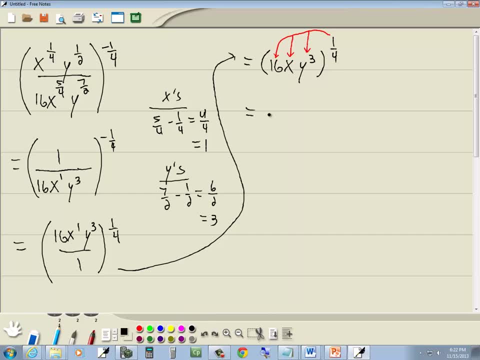 and we'll take the y to the third to the one-fourth power. So we've got sixteen to the one-fourth, we've got x to the one-fourth and we've got y to the third power raised to the one-fourth power. 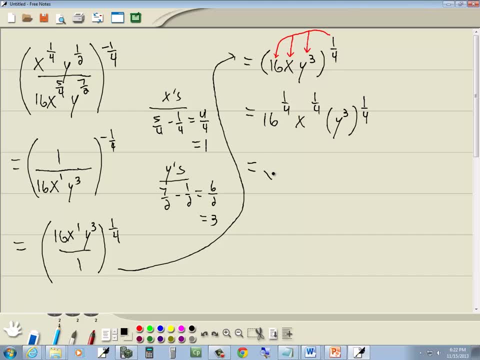 Now, sixteen to the one-fourth power is the same as the one-fourth power, Sixteen to the one-fourth. I'm going to put that back in a radical form. That would be the fourth root of sixteen, And then we've got x to the one-fourth. 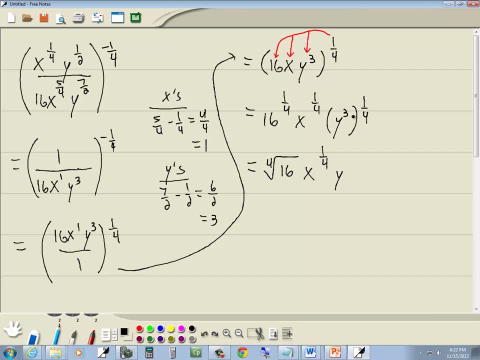 Now, when you're raising one exponent to another exponent, you multiply the exponents Three times one-fourth, gives you three-fourths, Now sixteen. if I do, the prime factorization of it is two times two. well, four, twos.